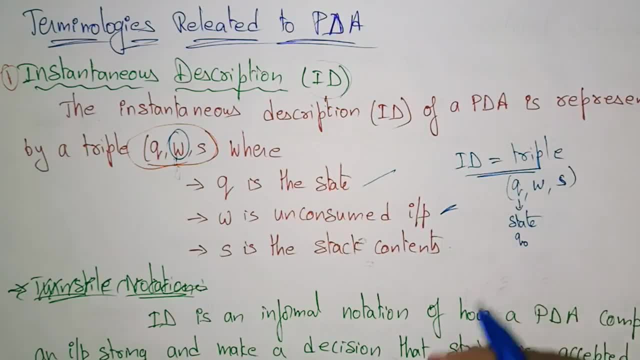 the initial state means: right, it is a Q. naught If you are start. next, If the state is changing means you have to write it as a Q one, like that. Okay, the start. this is the. it represents a state now coming to WW in the left hand side, So the left hand. 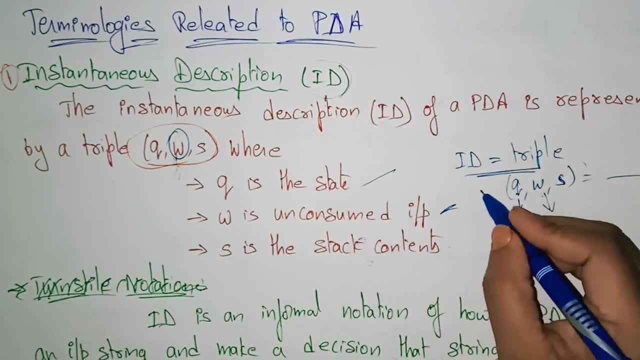 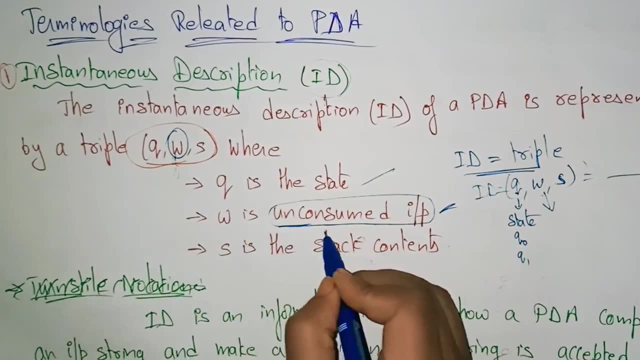 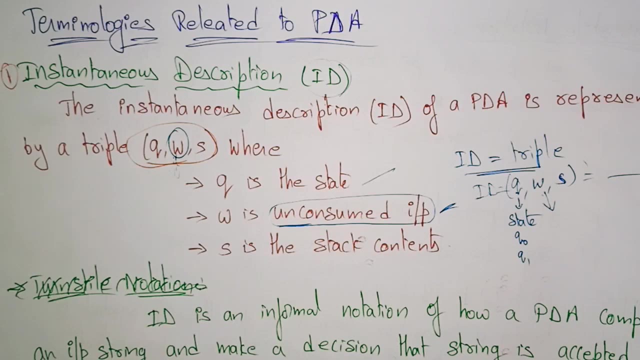 side and the right hand side will be there, but the left hand side you represent It is as an ID. Okay, so this W is nothing, but I'm consumed Input. Unconsumed input means still, you are not read. We didn't read that complete data that the finite state mission is not. 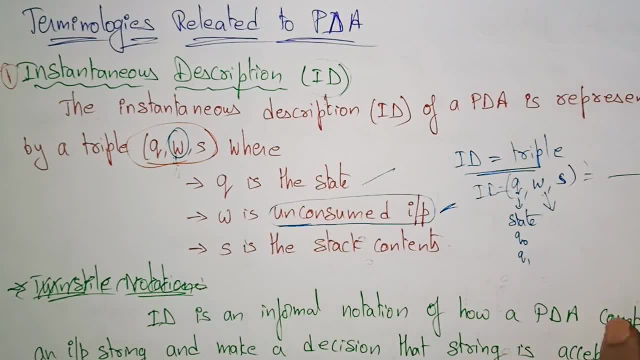 read data, that is, whatever the data that is present in the input stack. so in this you have seen in the diagram, okay, in the previous diagram, uh, the fine pushdown automata is consisting of three, uh, divided into three parts. okay, one is the finite state, finite control unit and this 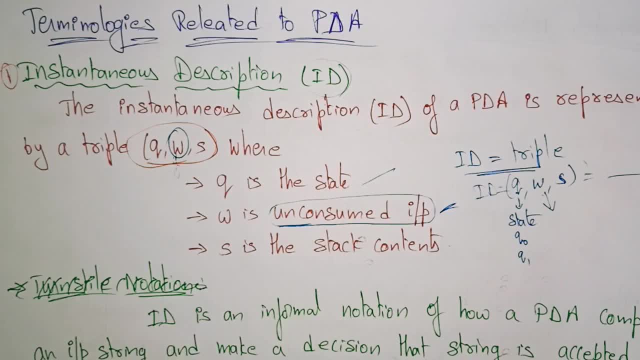 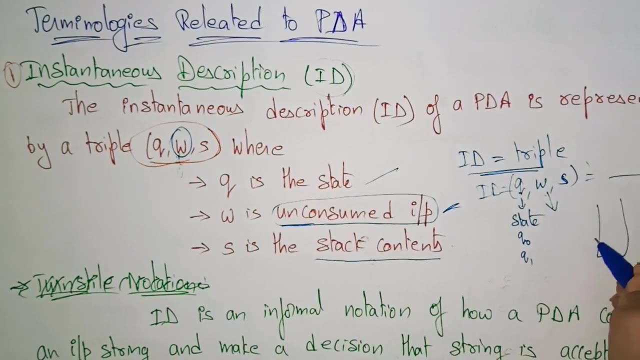 stack and the input tape. okay, input tape will be there so that, uh, input, consisting the tape, consisting of the unconsumed input, first, that is a w and s is the stack content. so, what is there in the stack, starting, whatever it may. next, what is the top of the stack? next, what element is there? 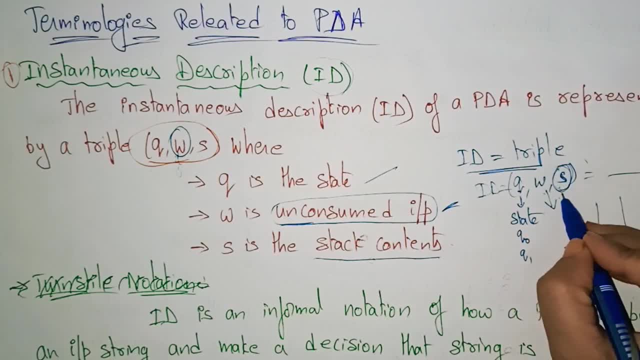 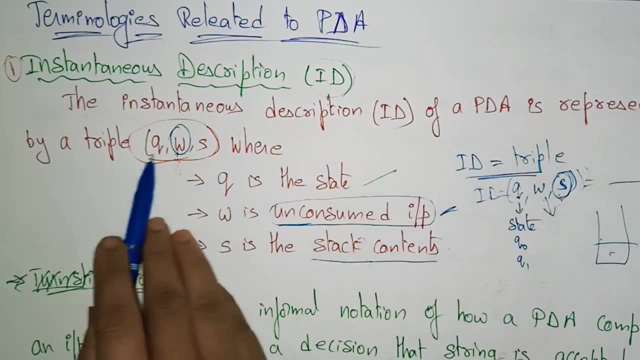 in the stack. so the elements that are present in the stack that you have to write here. this is a representation of id. the instantaneous description of a pushdown automata is represented by a triple. so remember this triple that is. this is the format is like this: only first the q has to be right that. 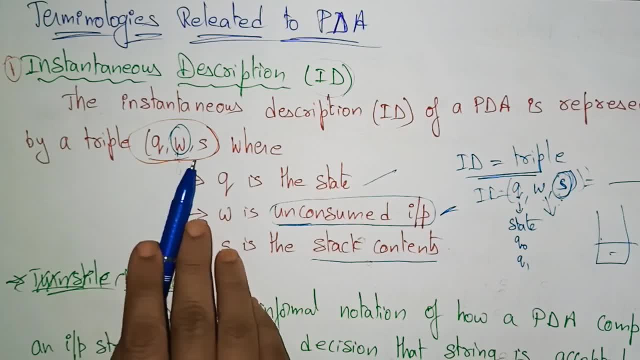 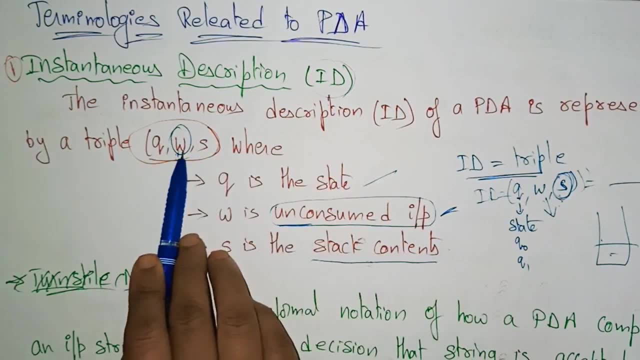 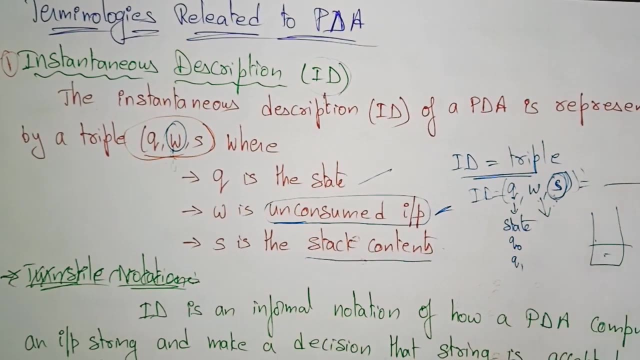 is a state and w that is a unconsumed input and s is a stack content. suppose whenever. if i write in the problems, if it is represented in three state means. that is nothing, but it is an instantaneous description. you are writing for that given grammar, for the given grammar, you have to write. 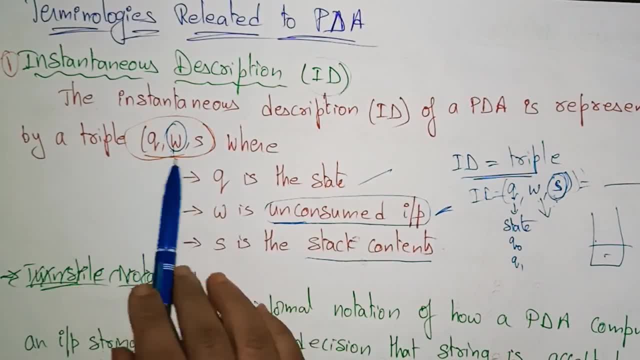 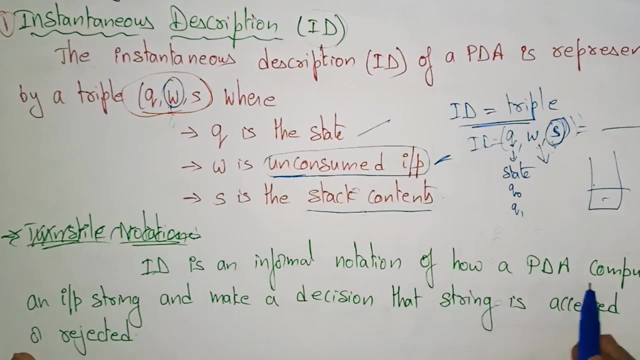 represent that, uh, that grammar in this. three triples. okay, in triples, remember this: q, w, s, q is a state, w is the unconsumed input and s is a stack content. suppose whenever, if i write in the problems, if it is an unconsumed input and s is a stack content. so here id is informal notation of how a pda computes. 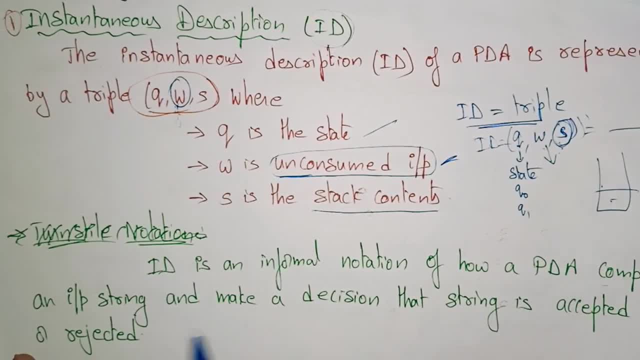 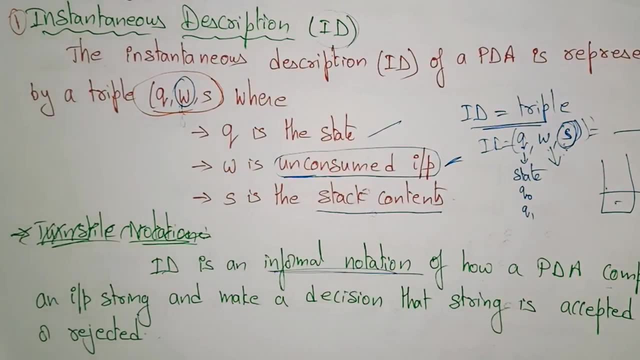 an input string and make a decision: that string is accepted or rejected. actually, this q w s is informal notation, not as a formal notation. just for the sake of solving the problem whether the string is accepted or rejected, the pda has to compute the input string, whatever the input. 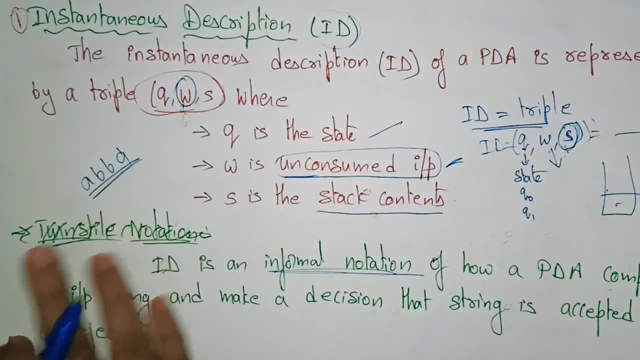 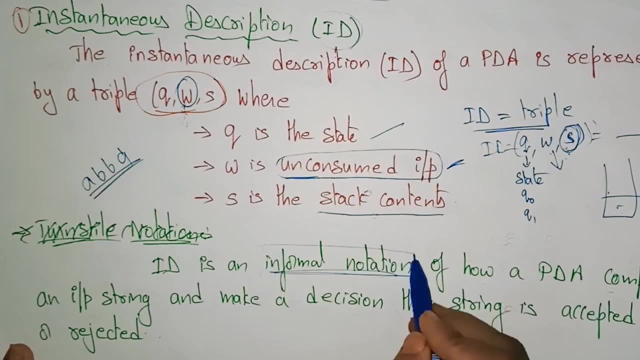 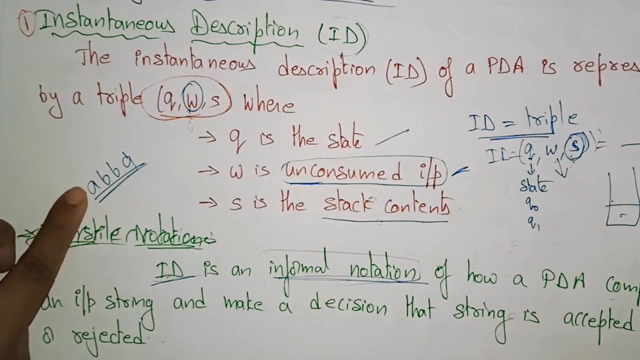 string. suppose a, b, b, a. this is the input string we are given. so this input string is accepted by pda or not. that decision has to be taken. that by using this informal notation id, with the help of this informal notation id, the pda is going to compute this input string and makes a decision. 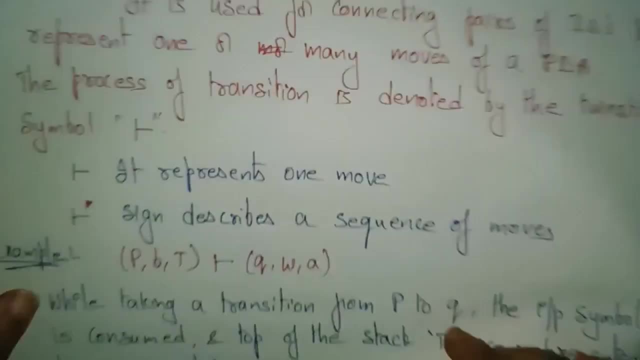 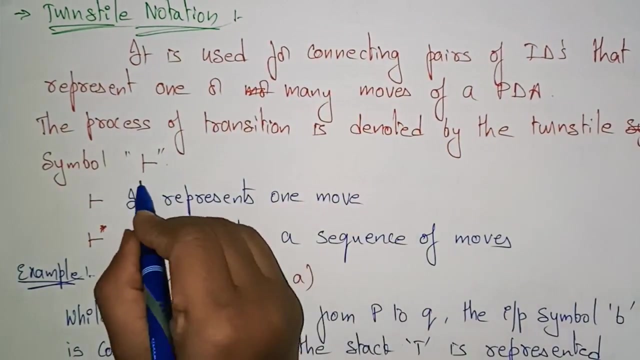 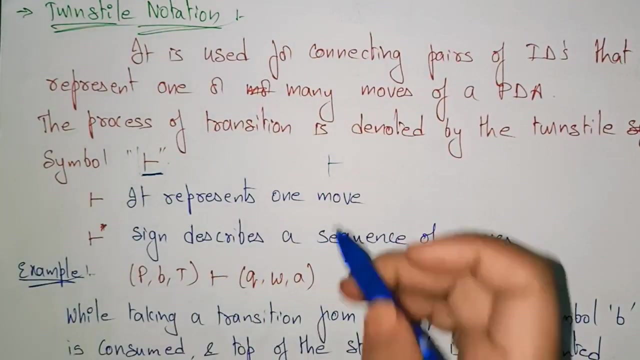 that string is accepted or rejected. so that is one terminology. and next, coming to the other terminology, that is a term style notation. so this is the representation of term style notation. just like the, the t has to be in like this: it should be converted: okay, it is fallen t. you call it as a fallen t. let's take it is used for. 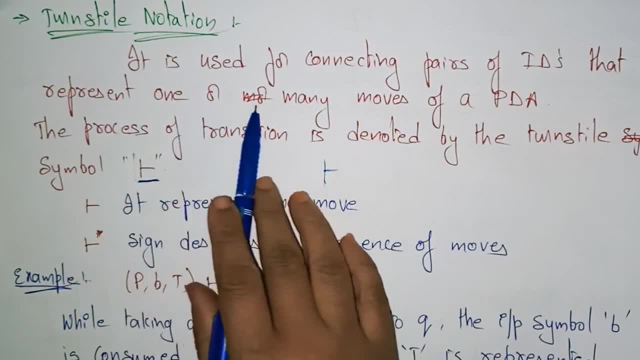 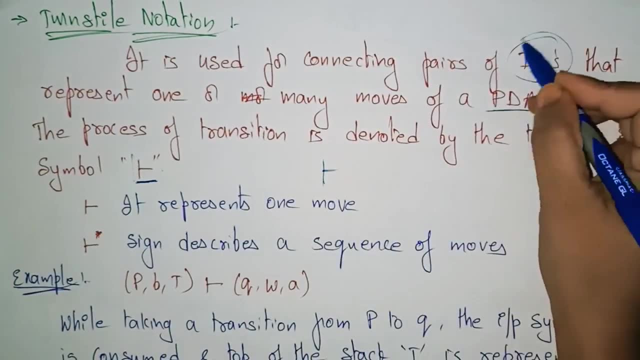 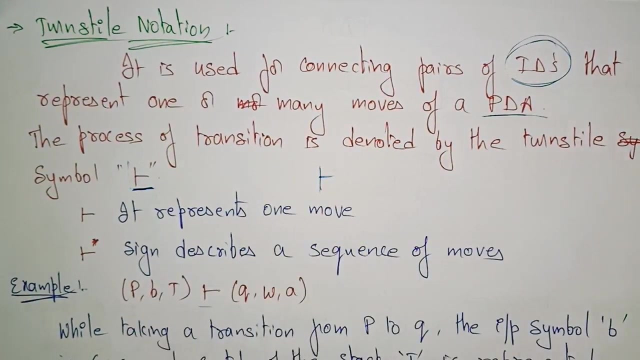 connecting pairs of ids that represent one or many moves of a pda. so the term style notation is used for connecting pair of ids. the pair of ids will be there. suppose two ids will be there. pair of ids has to be connected by using this. so here uh. 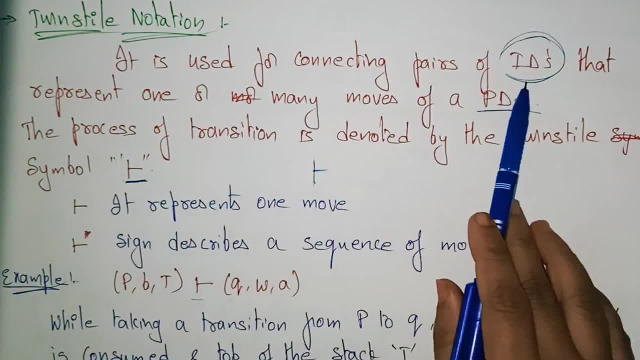 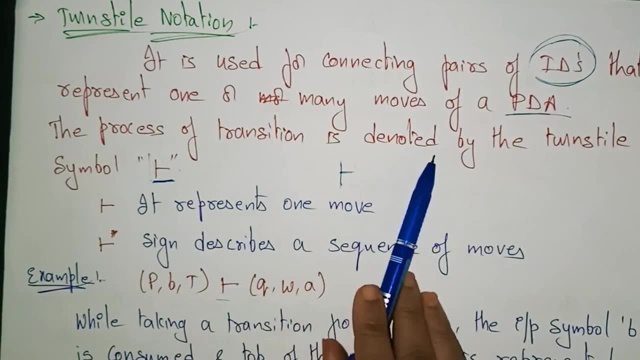 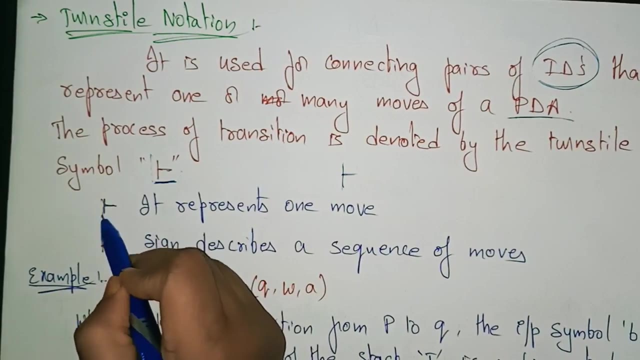 term style notation is used for connecting pair of ids that represent one or many moves of pda. so the process of transition is denoted by the term style symbol. so this is a symbol. so this is represents one move, suppose if only one is there. oh okay, only one move has to be taken. means from: 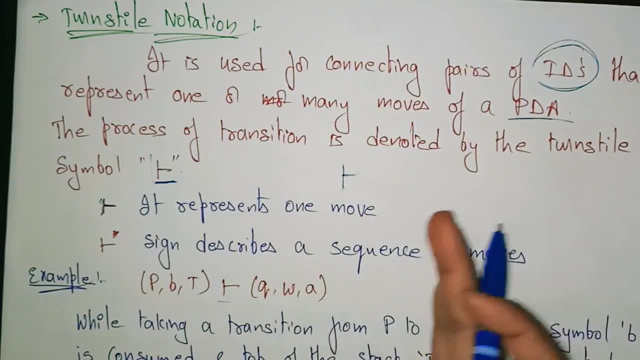 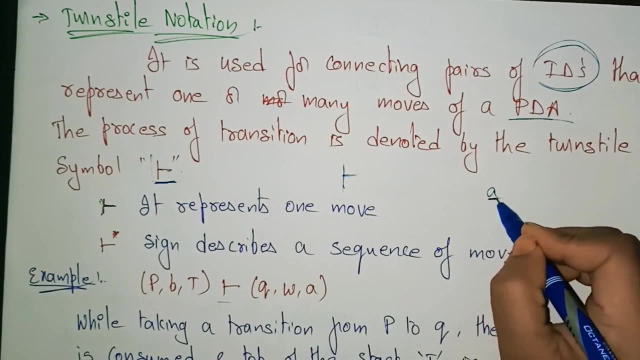 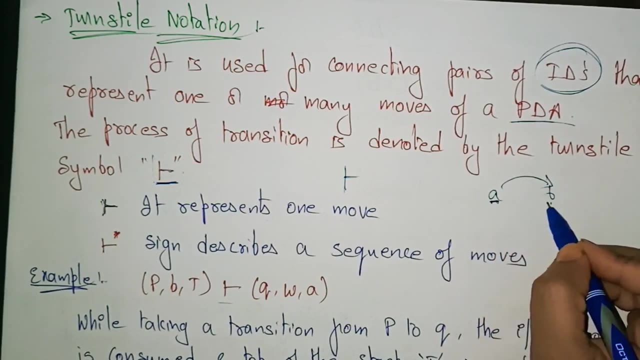 one state to another state. whenever a state is changing, that means the input symbol is changing: uh, from a to b. suppose you are reading starting. you are uh, in a, your read a and now you want to read b means the state the input symbol is changing. whenever the input symbol is changing, automatically the state has to be changed. 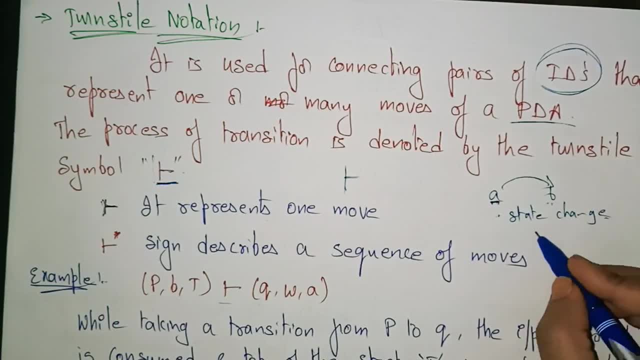 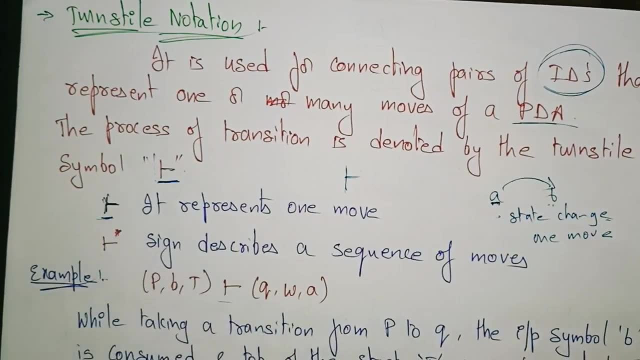 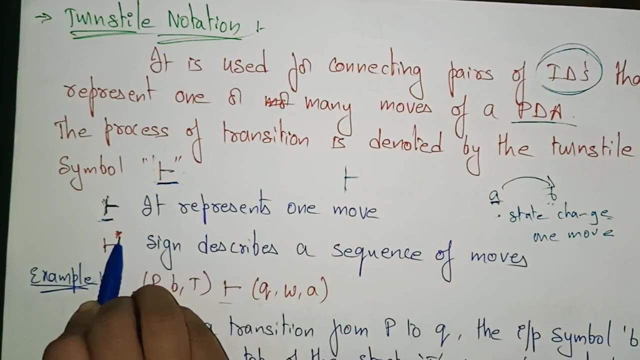 okay, the state has to be changed. that means one move has to be done so that that will be. that move represents the term style notation. so here the sign describes a sequence of the moves. suppose if it is the term style symbol. uh, here the star is there.